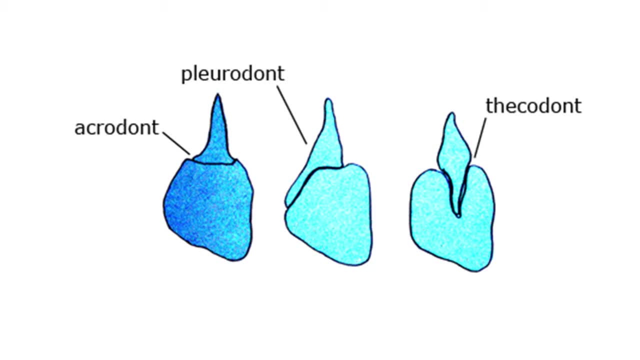 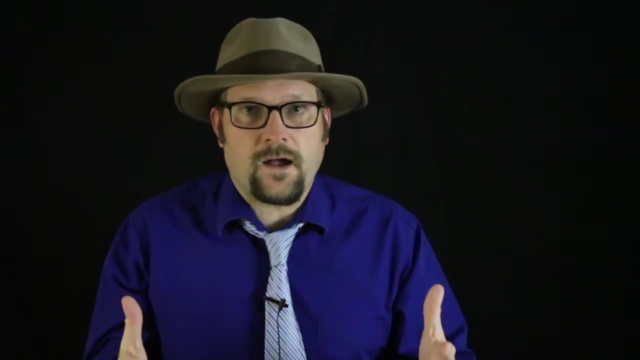 of the denarii and maxillary bones. These other conditions are found in the Lepidiosauromorpha, including in modern lizards. Early Archosauromorpha are historically called the thecodonts, because they all exhibit teeth. embedded in sockets, although this condition is also found in the descendants, including crocodilians, dinosaurs and toothed birds. With the mass extinction at the end of the Permian period, the early Triassic saw the slow arise of these small lizard-like creatures. 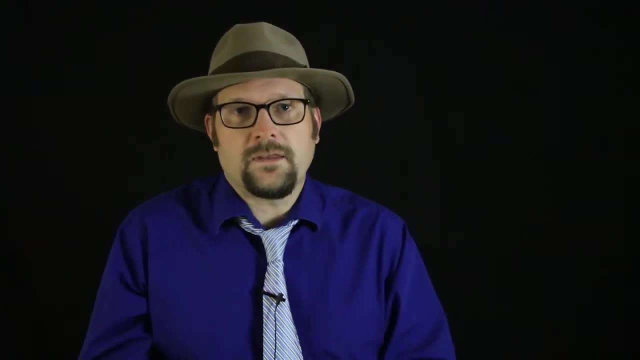 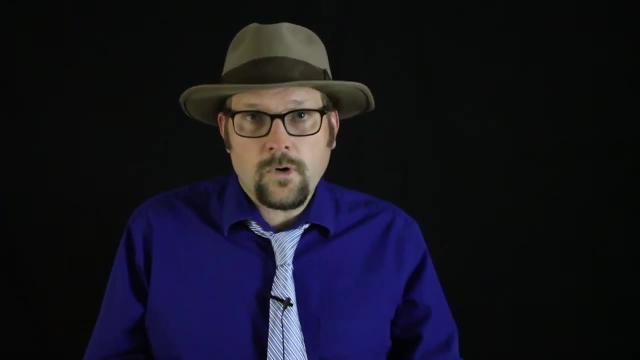 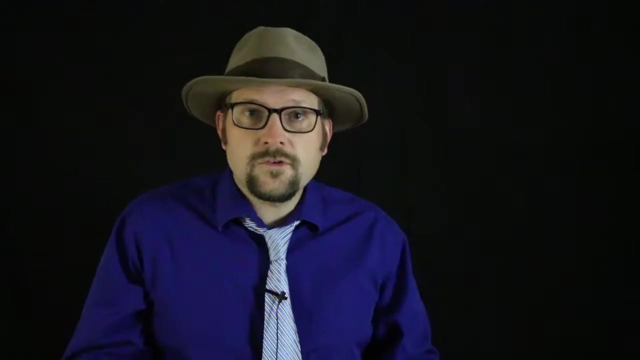 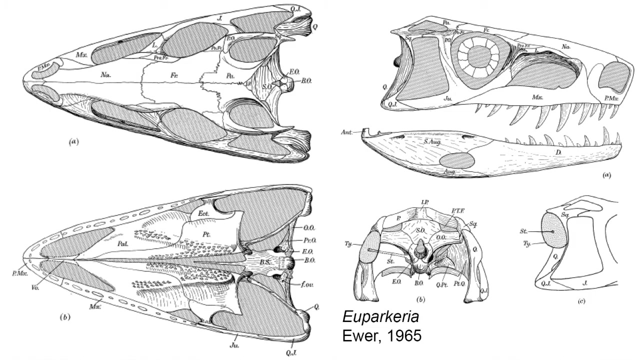 These creatures are now known as Euparkaria, which is known from South Africa. Euparkaria exhibits two additional features of the Archosauromorpha. Within the skull we see a new opening anterior or in front of the archosauromorpha. 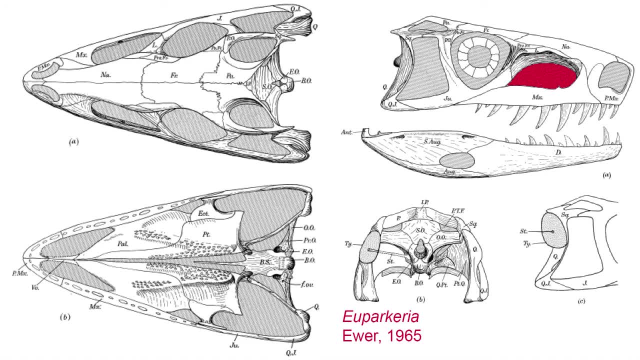 Euparkaria exhibits two additional features of the archosauromorpha. Within the skull we see a new opening, anterior or in front of the archosauromorpha, Between the lacrimal and maxillary bones. this opening is called the antorbital fenestra. 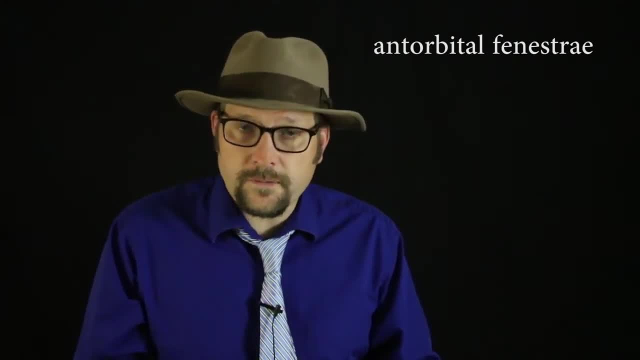 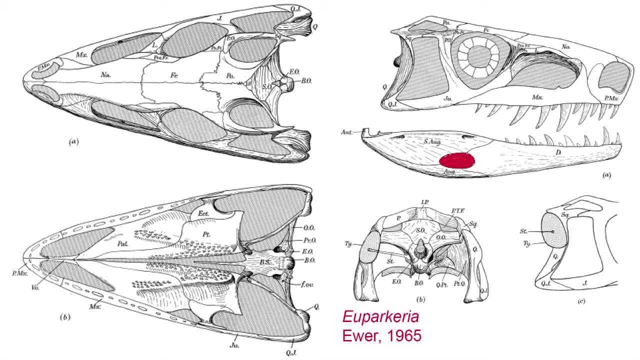 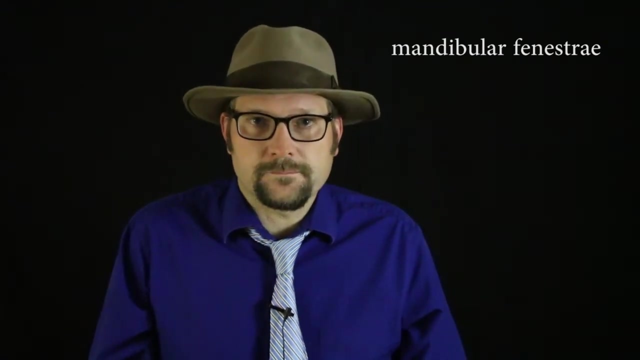 a feature unique to the Archosauromorpha. We can also see an additional opening in the lower jaw at the junction of the denarii superangular and angular. The opening is called the mandibular fenestra. Both of these openings can be found in later crocodiles. 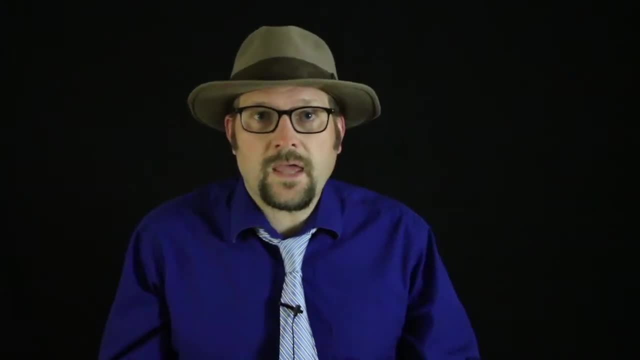 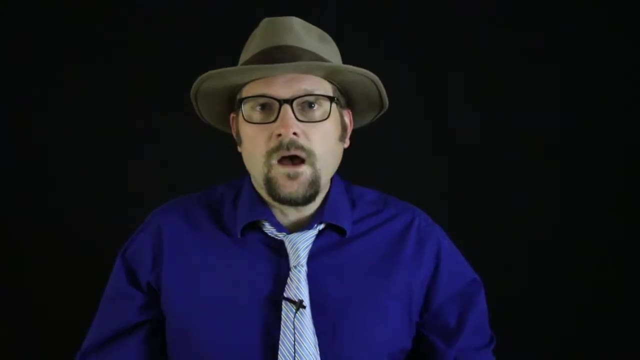 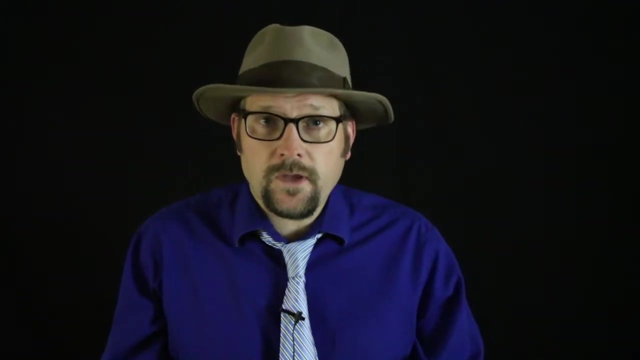 Euparkaria is a species of amphibians, pterosaurs, dinosaurs and birds, as well as a diverse group of archosauromorphans. Another key trait we see in Euparkaria is found in the two ankle bones, the calcaneum. 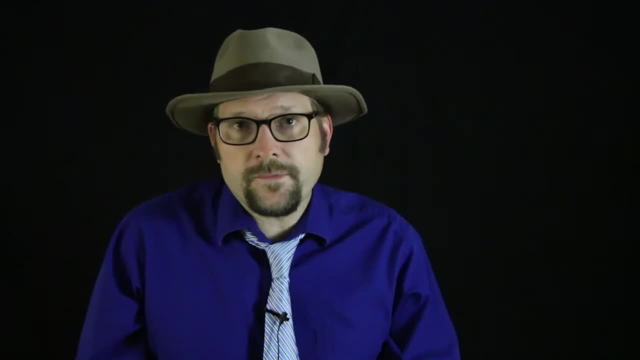 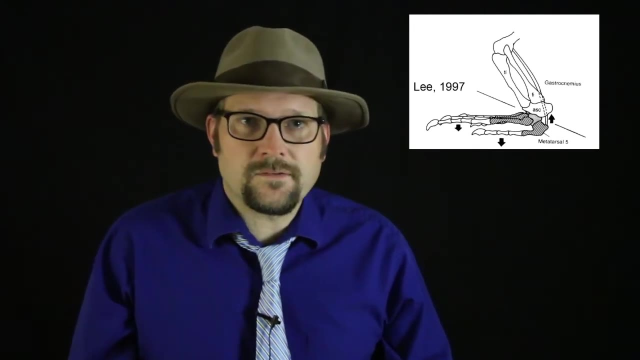 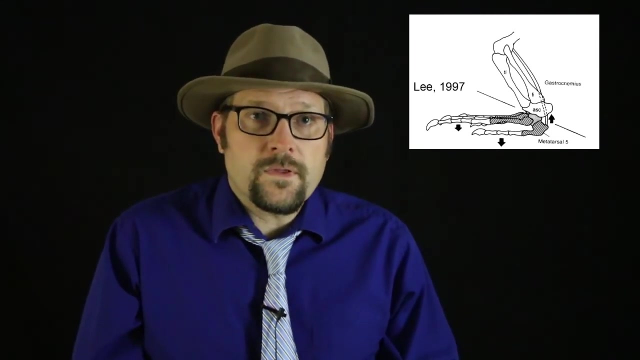 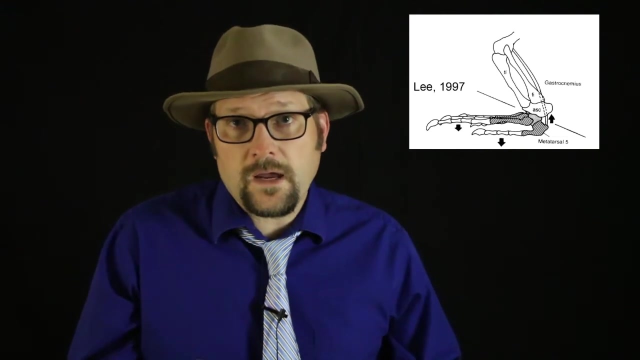 and the astragalus. In basal diapsids and in the Lepidiosoromorpha the two bones sit side by side, forming a, a broad bone that is often fused together in modern lizards, with the principal joint moving the foot between the fused calcaneum-astragalus bone and the metatarsal bones. 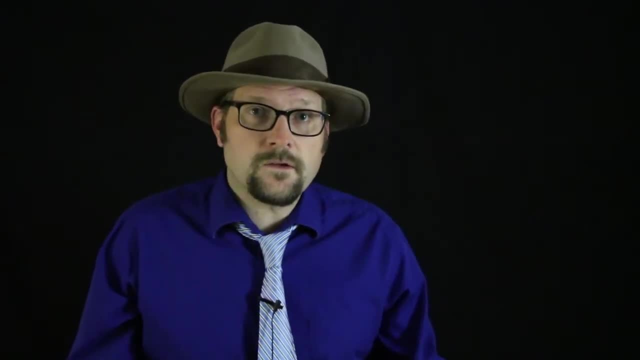 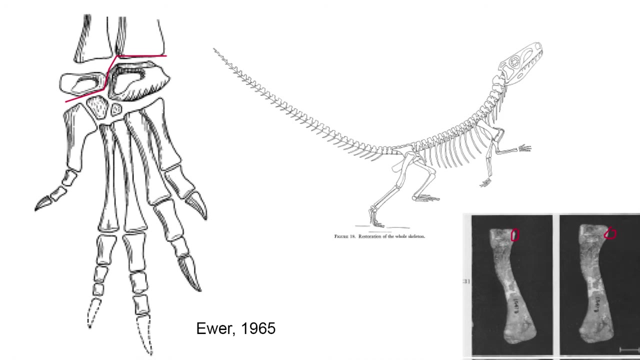 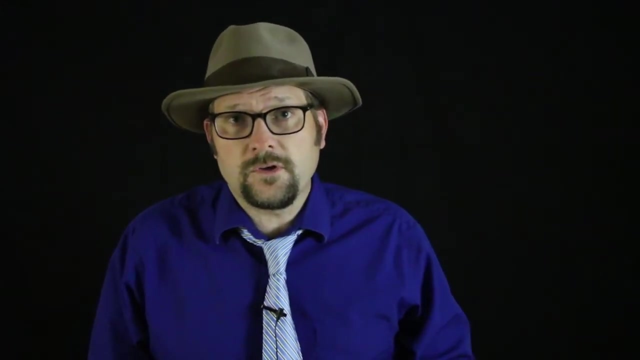 In Euparkaria, the calcaneum and astragalus form a joint between each other. This twisting joint allows the foot to rotate outward, which can help push the animal forward in running a sidekick motion to the hind leg. Some researchers have suggested that this joint was so well developed in Euparkaria. 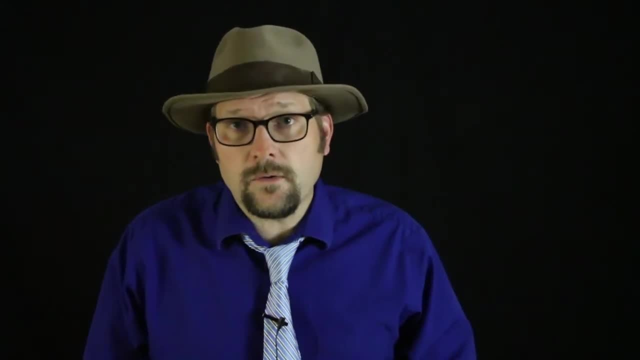 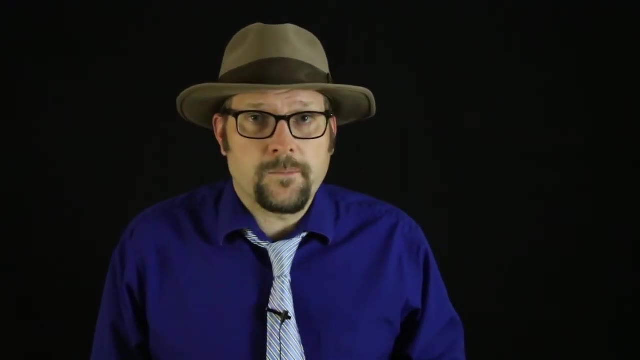 that it was able to support a semi-bipedal running pattern and some reconstructions of Euparkaria have it as a bipedal animal. It was a bit of a surprise to find out that it was a bipedal animal. 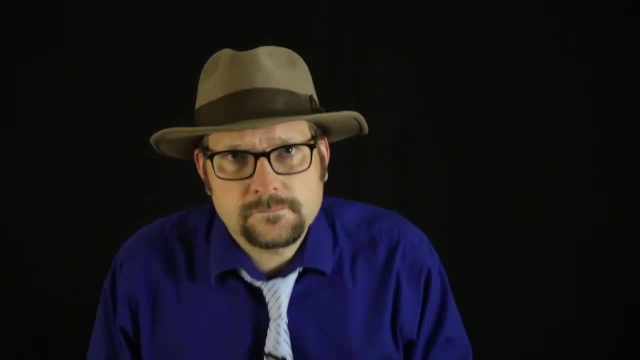 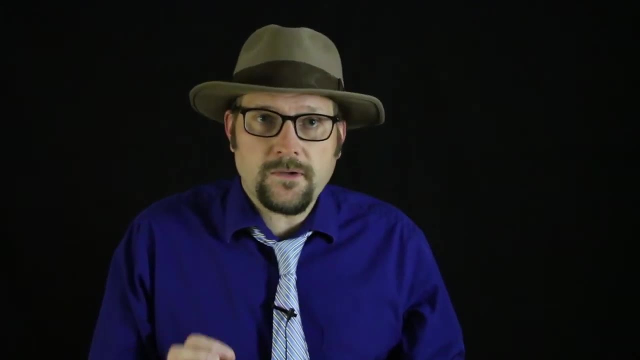 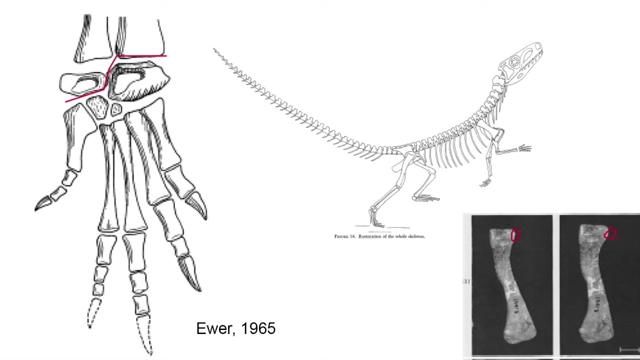 It was about the size of a small iguanid lizard. Euparkaria also had a well-developed, impedance-matching middle ear with the stapes bone supporting a tympanic membrane and housed in an air-filled middle ear chamber. The femur exhibits a protuberance called the fourth trochanter, which supported a large 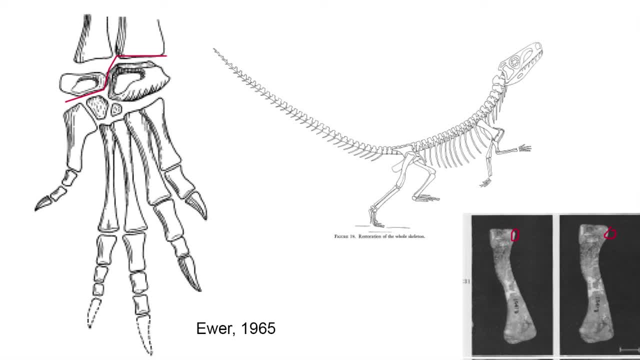 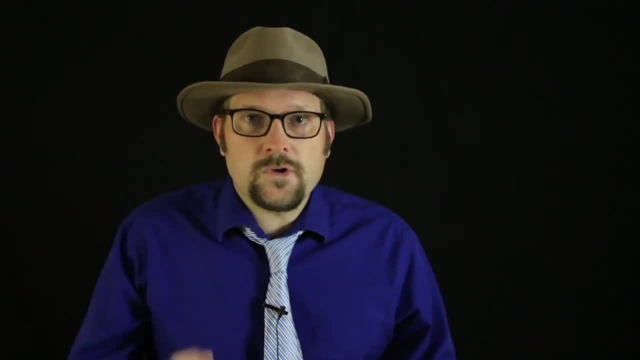 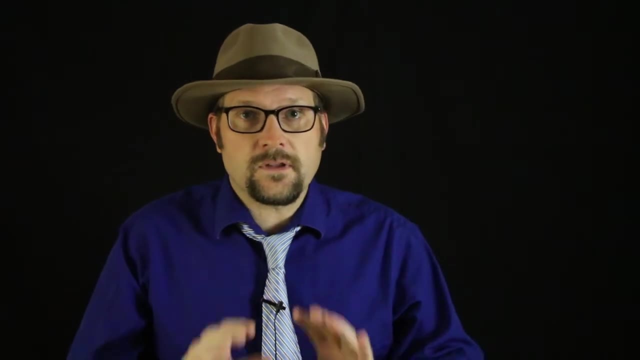 caudal femoris longus muscle. It ran between the femur and the caudal vertebrae which, when tensed, would retract the upper thigh. This fourth trochanter in the femur is a feature found in later dinosaurs which helps support. 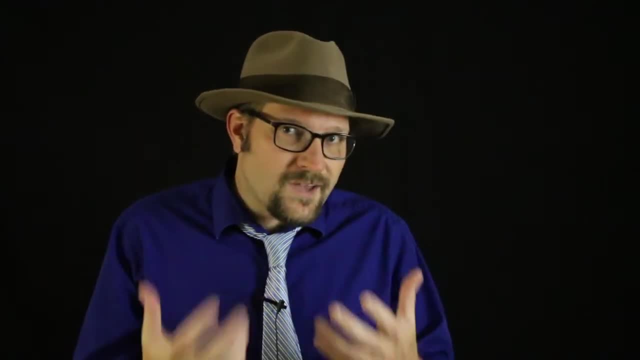 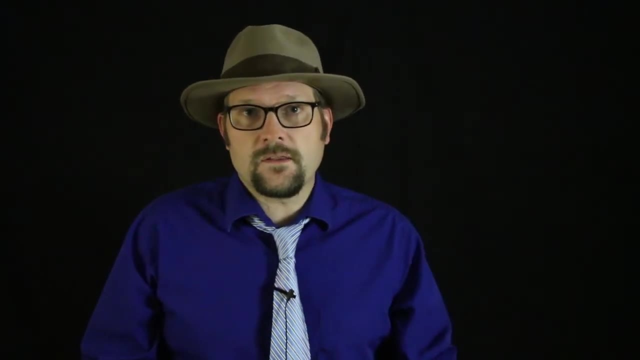 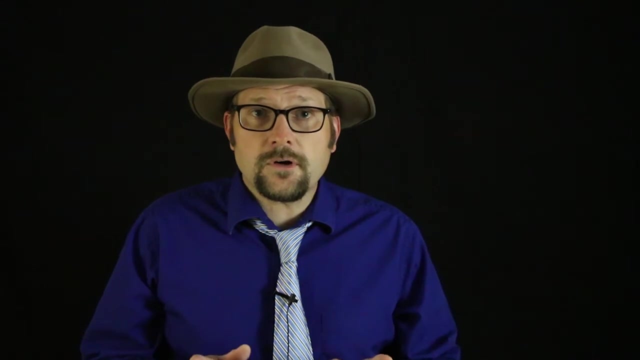 running and a more upright locomotive style. A final new trait we see in the archosauromorpha has to do with pneumaticity in the vertebrae and other bones. This is a feature that gives us a glimpse at how these early archosauromorpha breathed. 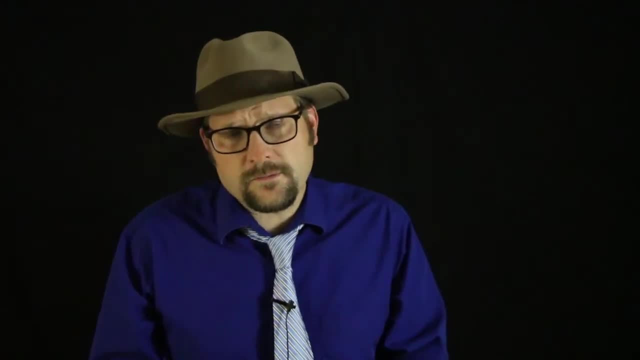 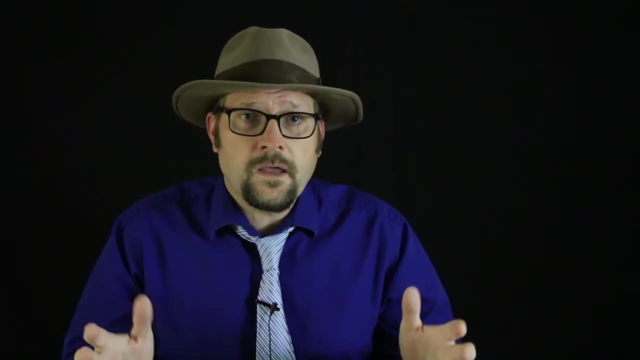 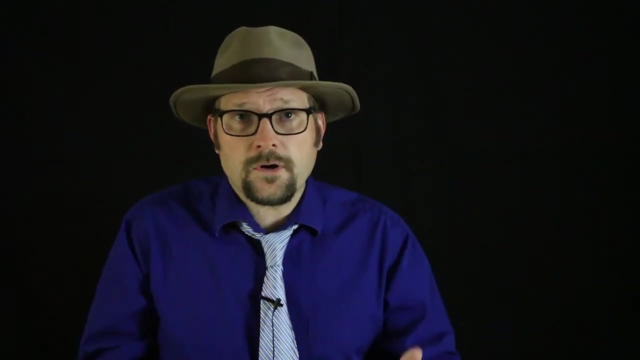 differently than most terrestrial tetrapods. In the next video, we will explore this pneumaticity across archosauromorphs and its importance in the development of a new style of respiration that is found in birds, dinosaurs and other dinosaurs and many primitive archosauromorphians. 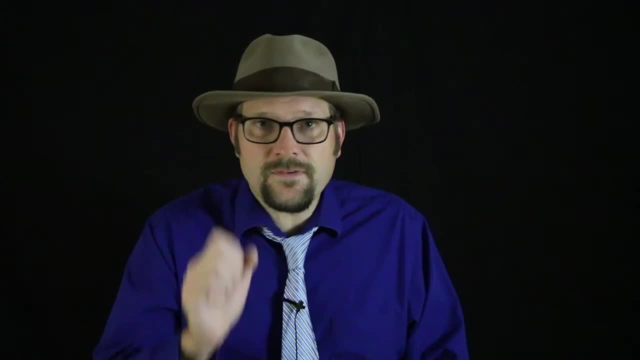 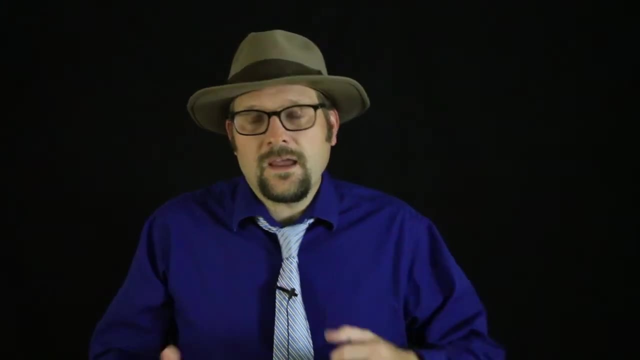 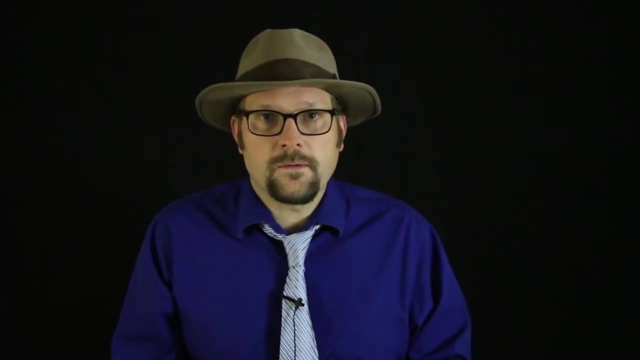 For now, be sure to review the key features of basal archosauromorphs and be able to identify them on a skeleton and skull: The thecodont teeth, the anorbola fenestra, the mandibular fenestra, the fourth trochanter.